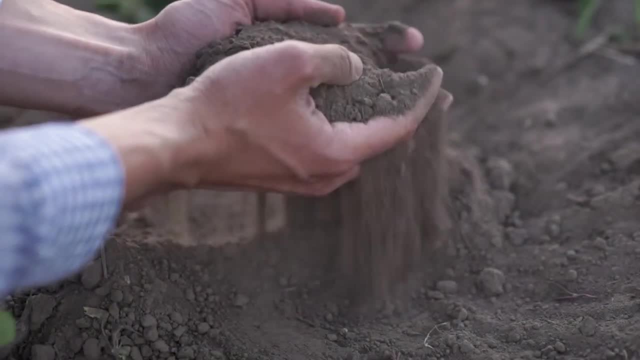 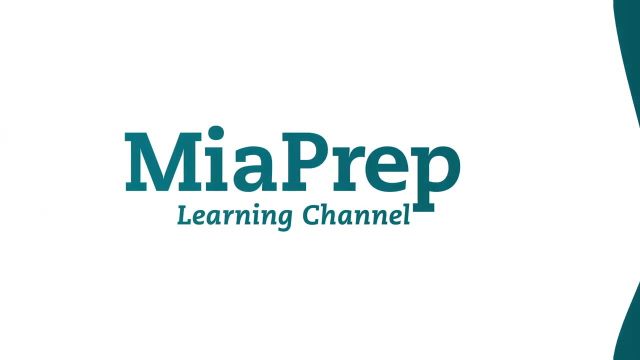 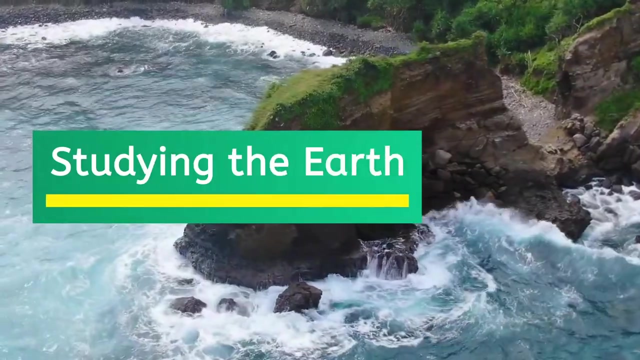 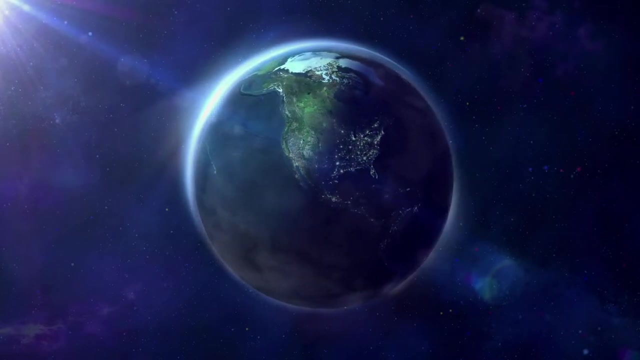 So today we'll begin a brief journey into the world of geography. Ready explorers, If we want to study the Earth, we should know what it's made of and how it works Before we begin our study of the land and water. pause the video and show what you know. 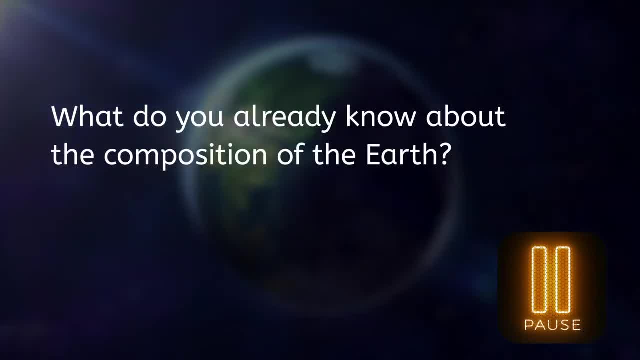 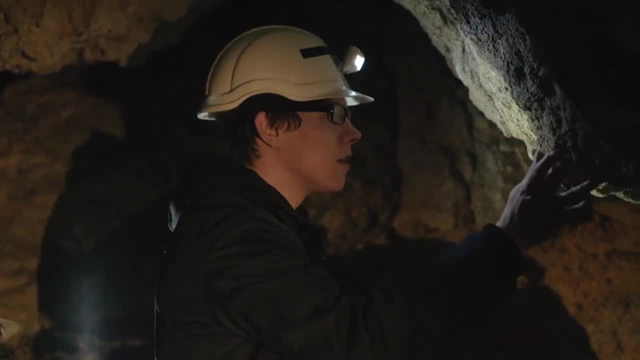 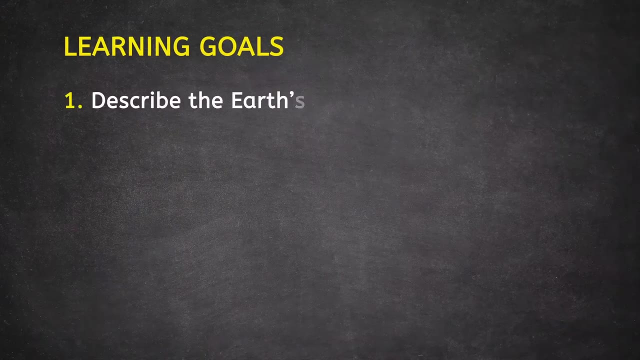 in your lesson guide 1.. The people who study the Earth's physical structure and history are called geologists. We'll be taking a page out of their book as we learn about the land and water. Our learning goals are: to describe the Earth's surface, land and water composition. to categorize. 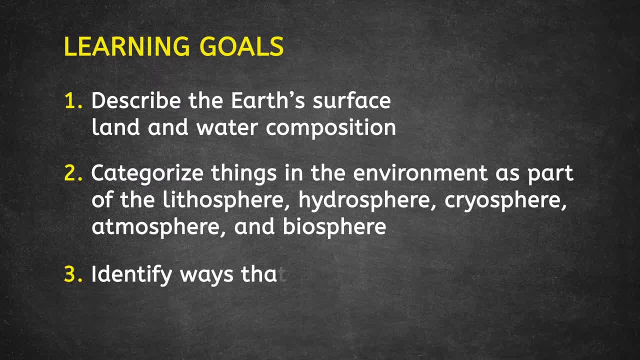 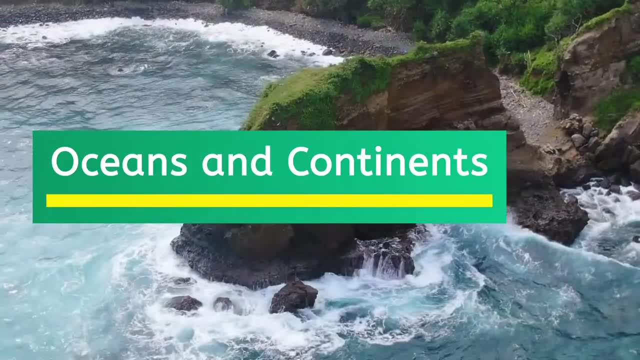 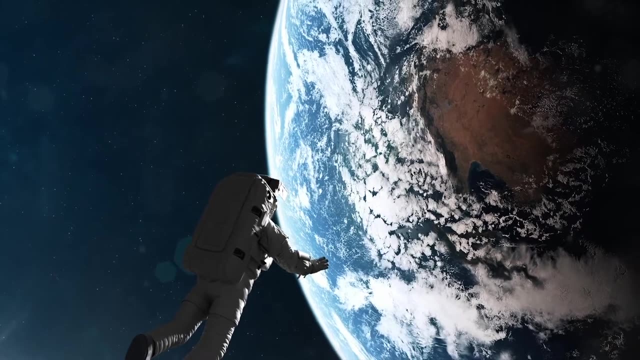 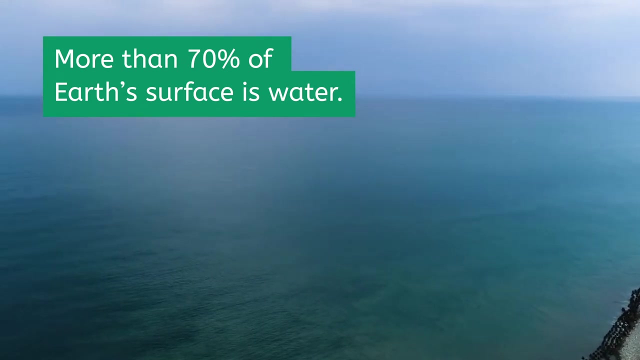 things in the environment into different spheres and to identify ways that humans interact with those spheres. If you were to fly up to space and view the Earth from afar, you'd quickly discover that it's a watery planet. More than 70% of the planet's surface is water, mostly saltwater in the form of oceans. 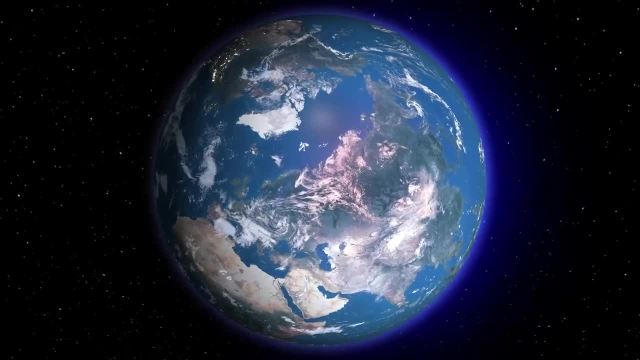 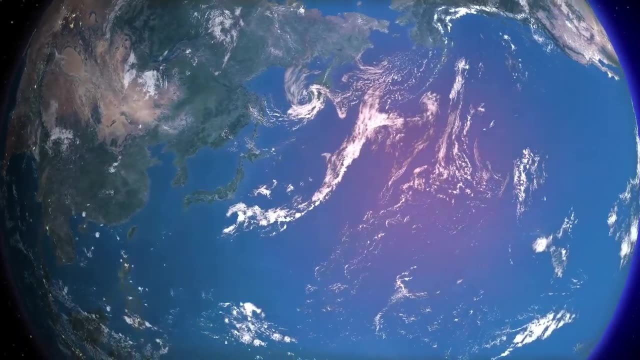 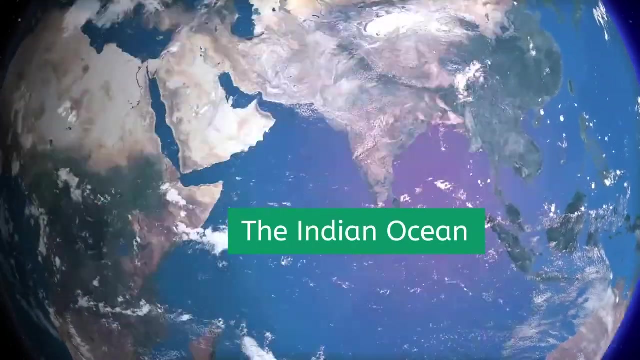 and seas. Do you know how many oceans the Earth has? Well, some argue that there's only one, an interconnected global ocean, but most countries recognize five named oceans: The Pacific, the Atlantic, the Indian, the Arctic and the Southern Oceans. 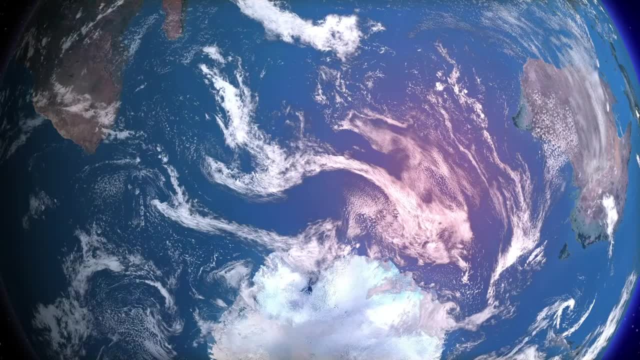 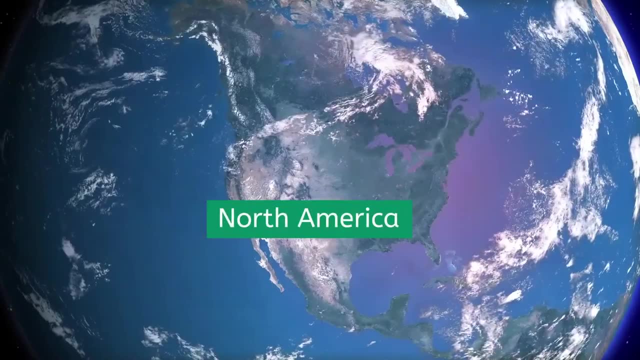 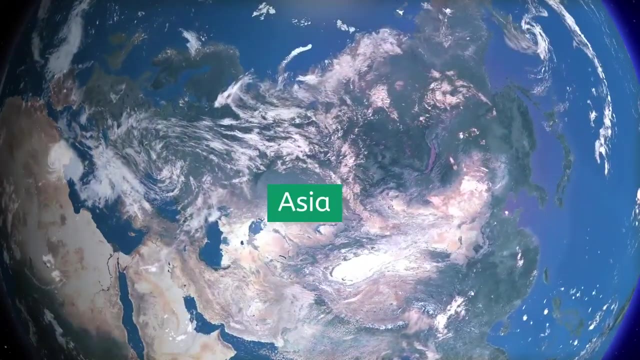 The large, continuous expanses of land that rise above sea level, separating those oceans are called continents, and there are seven of those- North America, South America, Europe, Africa, Asia, Australia and Antarctica. 2. The world's largest ocean. 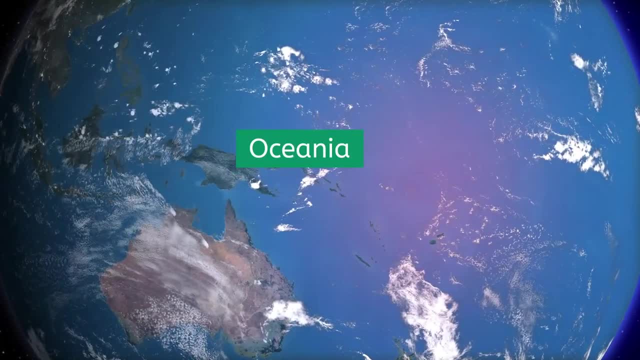 3. Sometimes an eighth continent, Oceania, is added to this list to account for the islands scattered across the Pacific. Most of the time, these islands are left off the list because they don't really meet the description of continuous expanses of land. 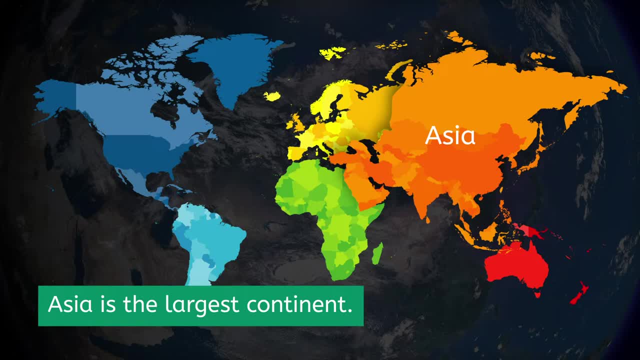 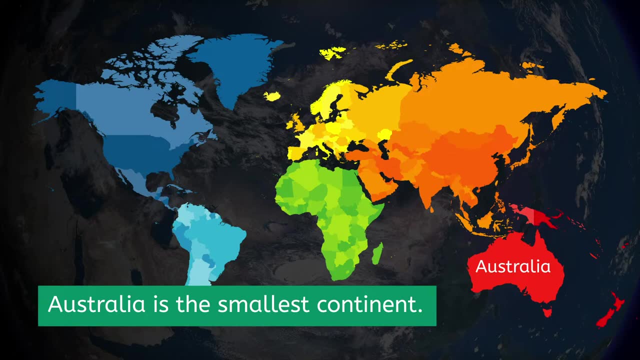 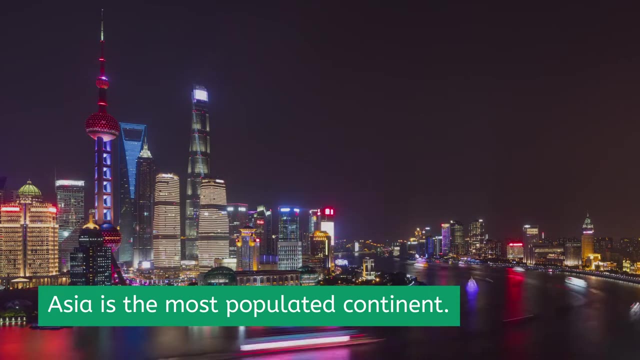 Asia is the largest continent by far, with 17.2 million square miles of land. Australia is the smallest, with just under 3 million square miles. Asia is also the largest continent in terms of population, hosting more than 4.4 billion people- over half the global population. 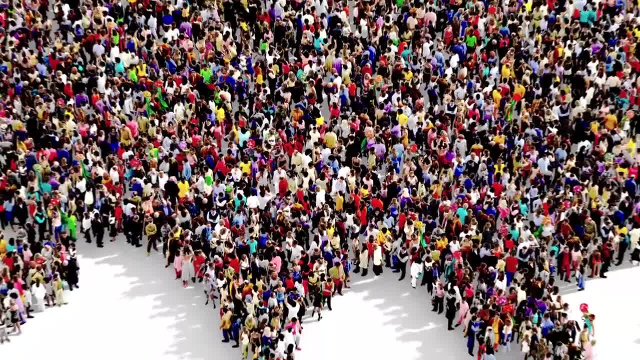 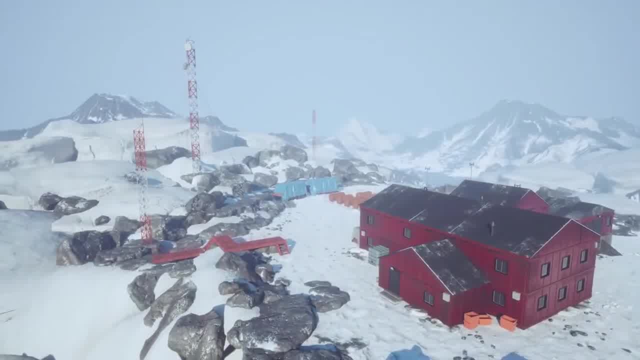 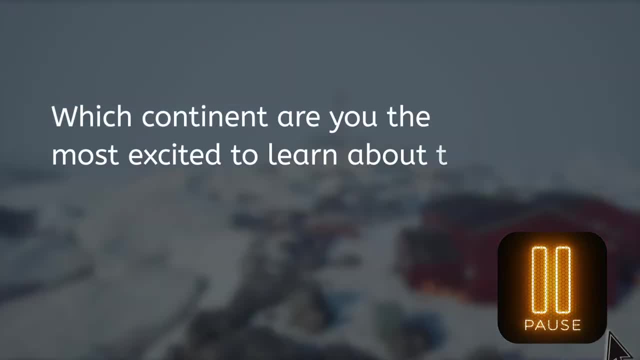 Estimates suggest that, of every human to ever walk the Earth, one out of 20 of them is living in Asia right now. The least populated continent is Antarctica, which has research stations but no permanent residence. Which continent are you most excited about? What are you most excited to learn about this year? 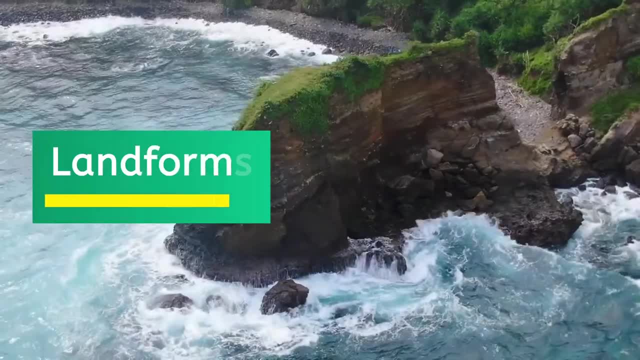 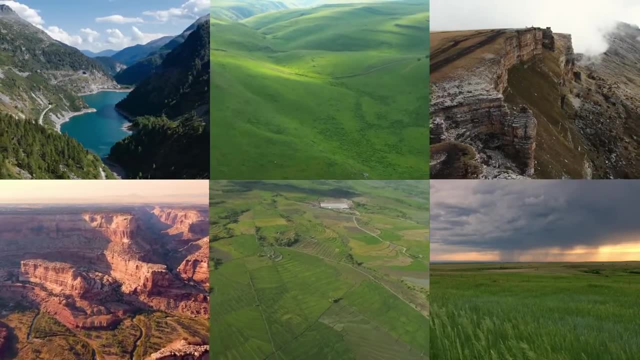 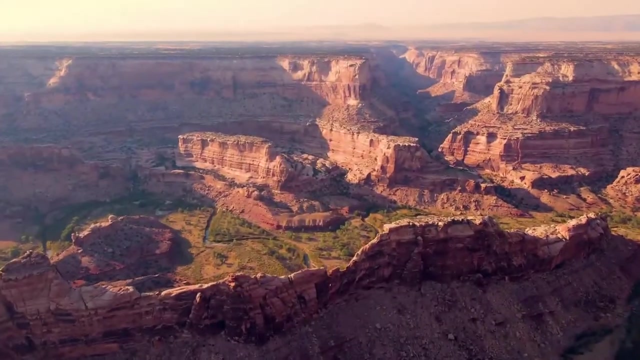 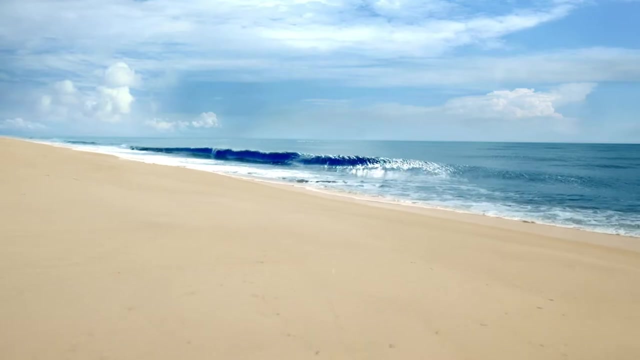 Respond in your PDF. Continents are made up of landforms, natural features of the surface of the Earth. A few examples include mountains, hills, plateaus, canyons, valleys and plains. Landforms can also include shoreline and submerged features such as bays, gulfs, peninsulas, seas. 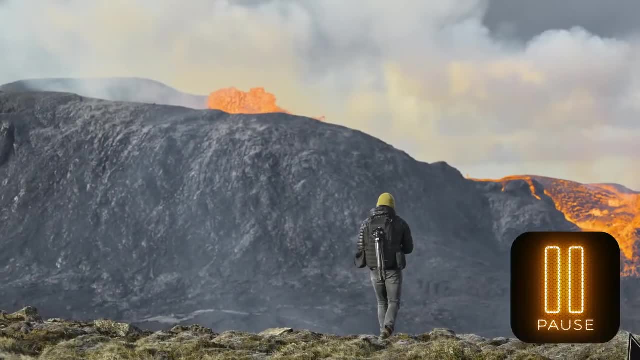 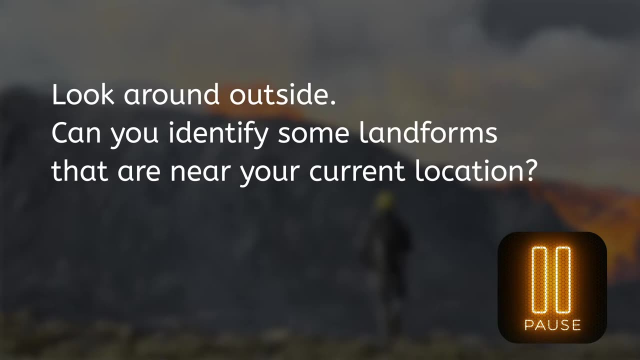 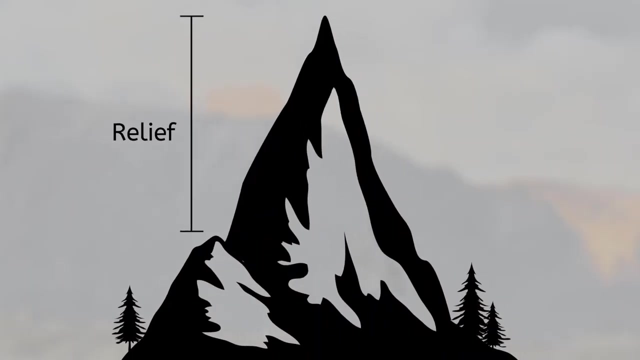 Can you identify some landforms that are near your current location? Pause the video, look around outside and see how many you can find. Typically, landforms are classified according to their relief, which is the difference in elevation between their highest and lowest points. 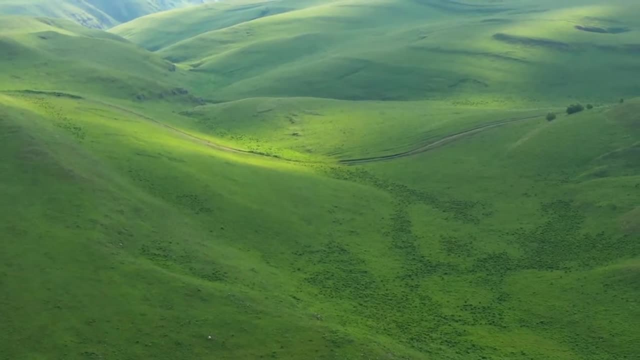 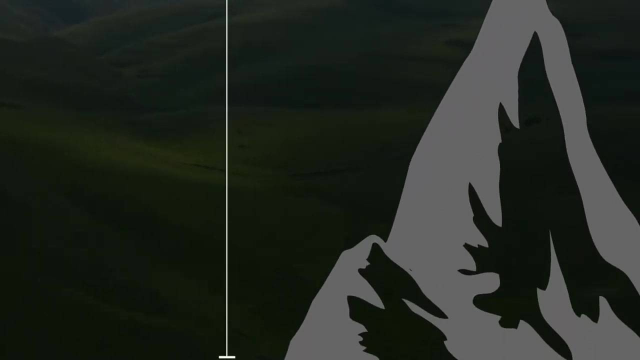 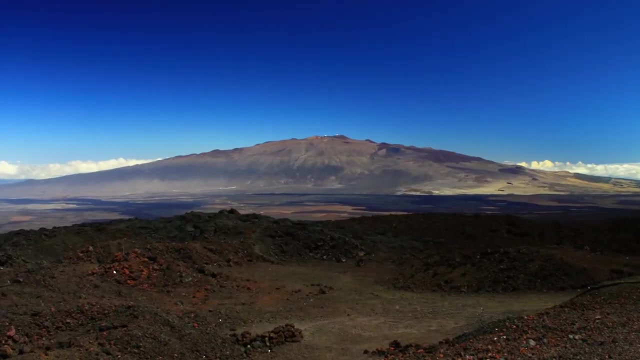 Mountains have high relief. Hills, which are typically lower and rounder, have lower relief. So what's the highest mountain in the world? Everest, right? Well, actually, no, It's Mauna Kea in Hawaii. Mount Everest stands at 29,031 feet above sea level. 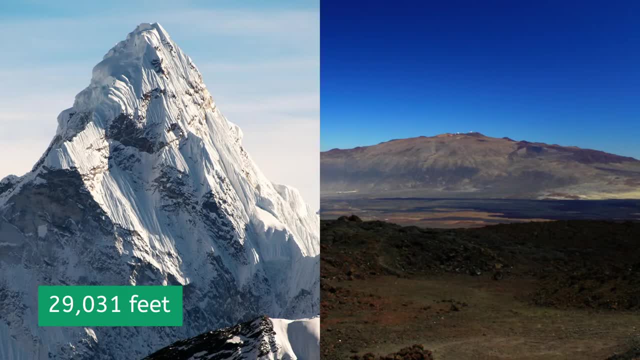 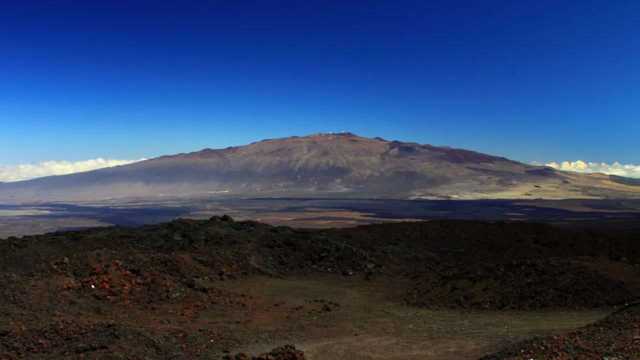 Very impressive. Mauna Kea, on the other hand, stands at only 13,796 feet above sea level, And yet it's nearly a mile taller than Everest. How is this possible? Well, Mauna Kea extends 19,700 feet below the ocean's surface. 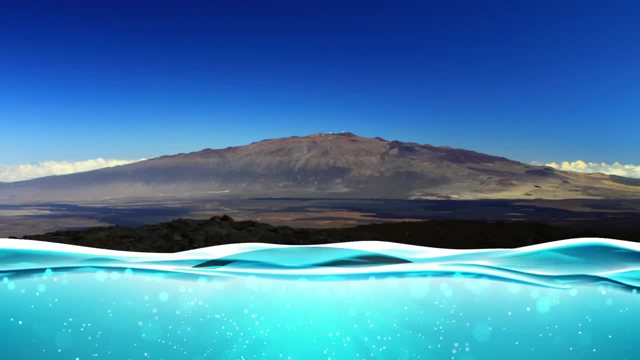 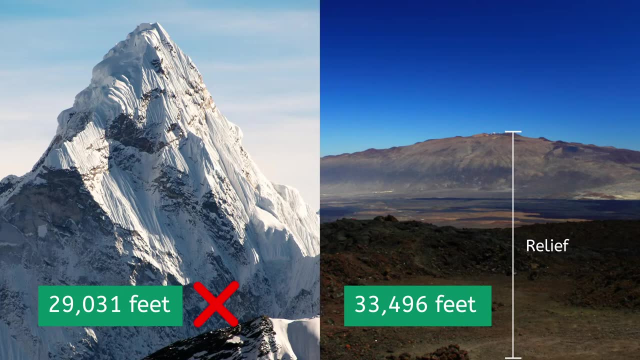 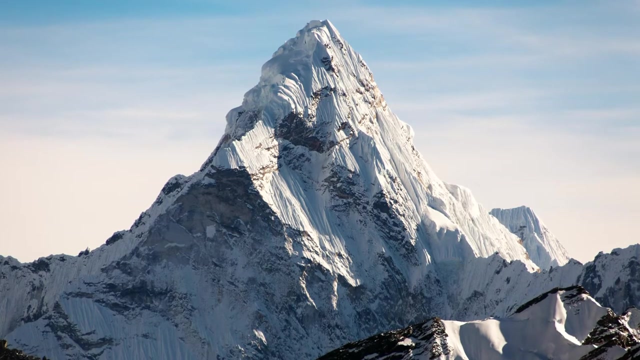 Over half of it is submerged in the waters of the Pacific. So if we measure it by relief, its total height is a staggering 33,496 feet. Now don't worry Everest fans: Mount Everest is still the tallest mountain on Earth in terms of altitude. 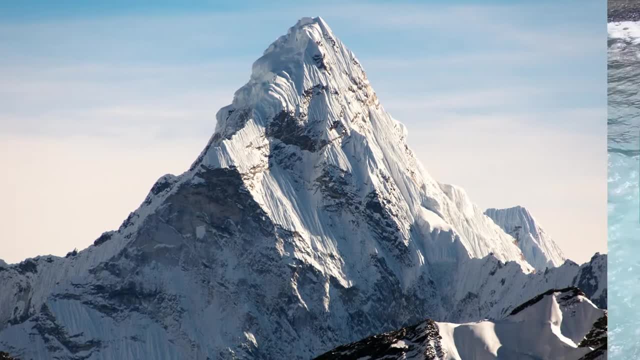 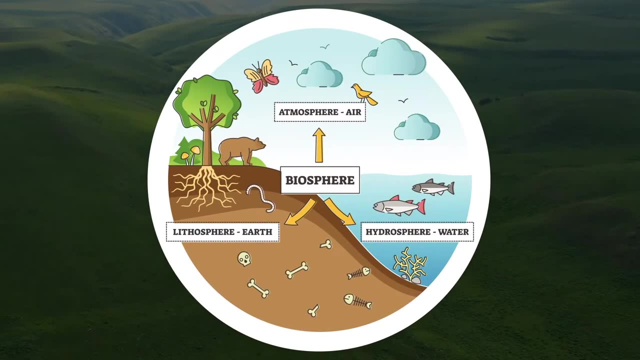 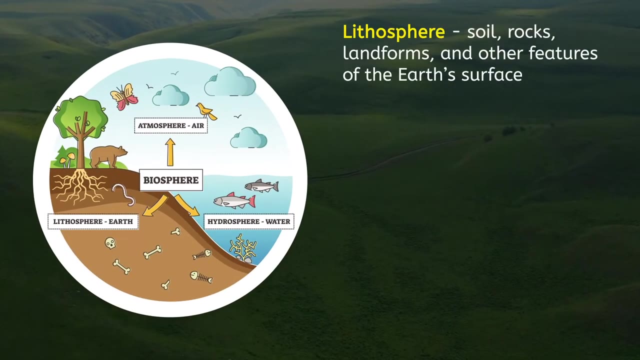 meaning the summit's elevation above sea level. The Earth's crust is composed of lots of different things classified into many spheres. Soil, rocks, landforms and other features of the Earth's surface make up the lithosphere. The air, water vapor and other substances above the Earth's surface make up the atmosphere. 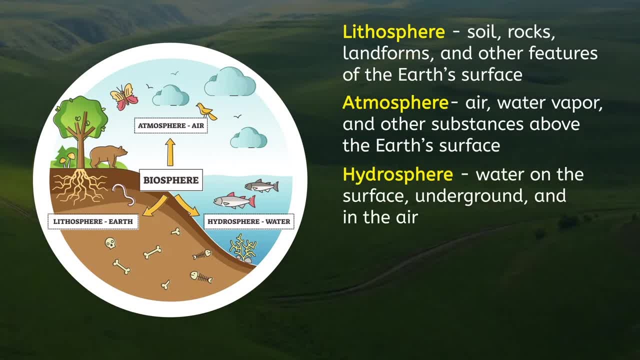 Water on the surface, underground and in the air makes up the hydrosphere. Sometimes the water is permanently frozen and you'll hear that part of the sphere called the cryosphere. And of course, the biosphere is made up of the parts where life exists. 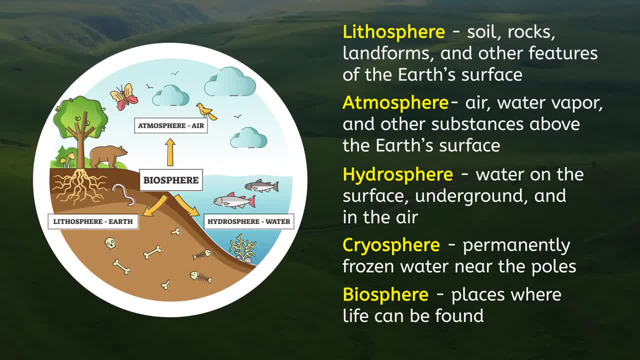 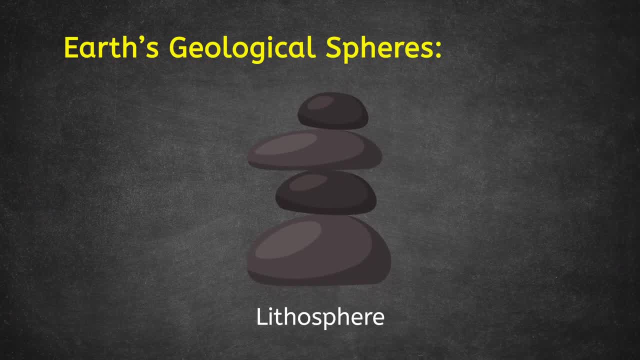 It's the world of plants, animals and other living things on land and in the water. That's a lot of Greek vocabulary, so let's break down those words. Litho means stone. The lithosphere is therefore the sphere where the rocks are. 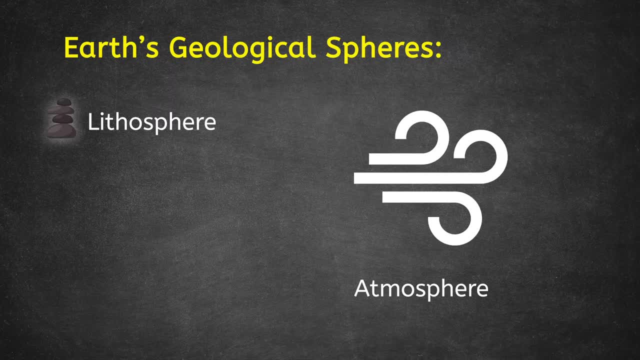 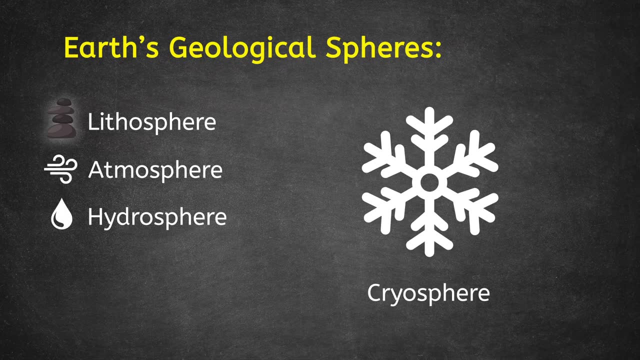 Atmos means vapor, so the atmosphere is the sphere where the air is. Hydro means water and cryo means frozen, so those are the spheres containing water and ice. And finally, because bio means life, the biosphere refers to where life is found. 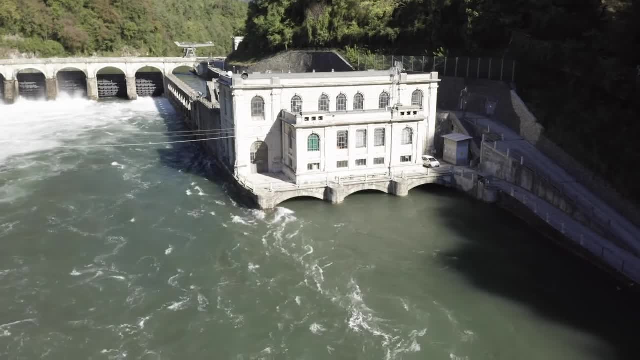 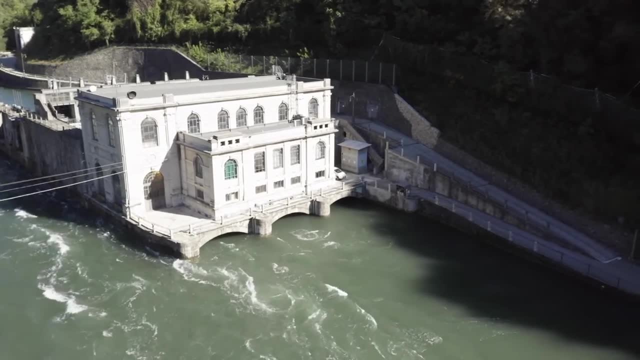 We'll look at interactions among the spheres as well. For example, humans in the biosphere might harness energy from the hydrosphere by having it spin turbines in the lithosphere to produce electricity. Check out the practice questions in the lesson guide. 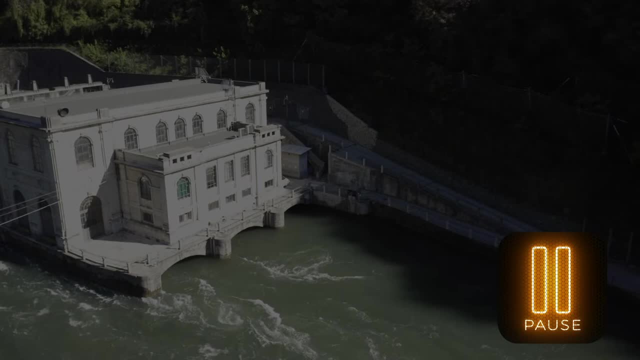 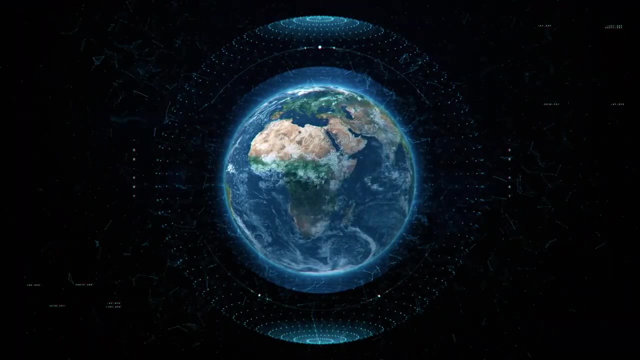 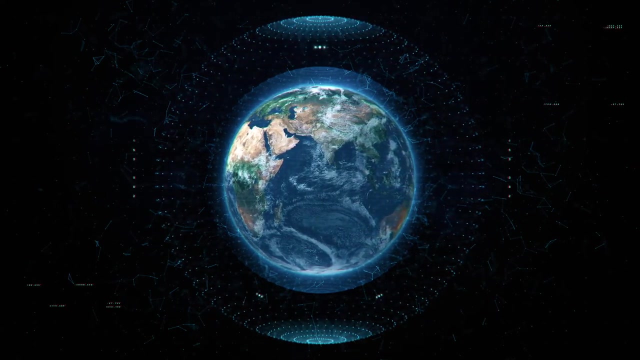 They will help you get more familiar with your vocab. Take a second to practice what you've learned. As we continue our study of geography, we'll need to incorporate an understanding of the Earth when we think about the people who live in it. In the same way an auto mechanic thinks about cars and how they're put together, I want you to think about the Earth and what it's made of. 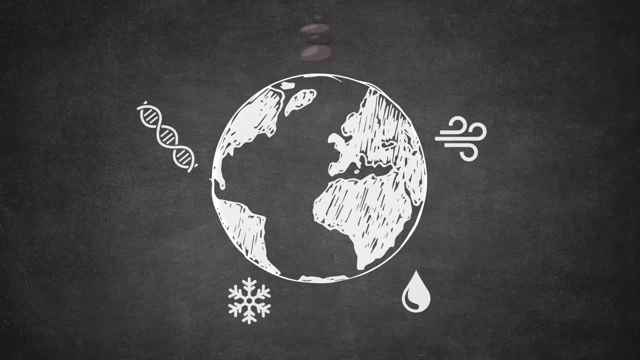 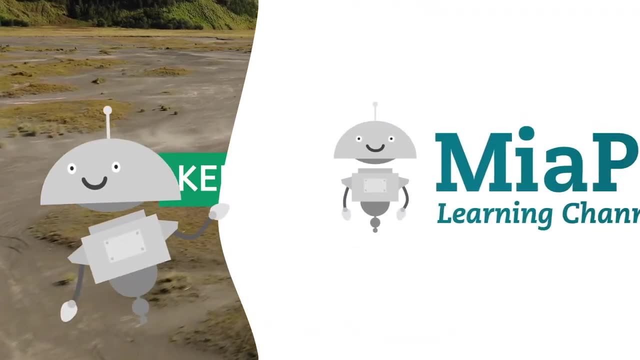 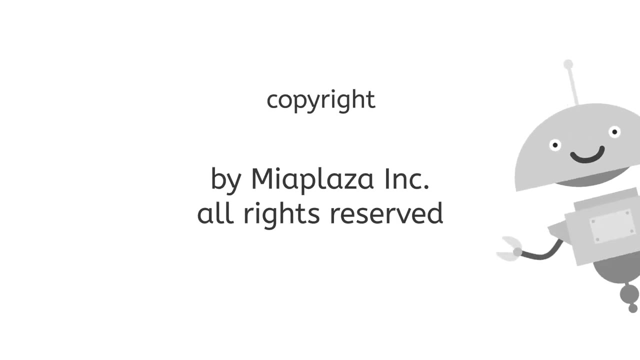 Challenge yourself to think about how land, air and water shape the world around you And until next time, keep exploring. NASA Jet Propulsion Laboratory, California Institute of Technology.